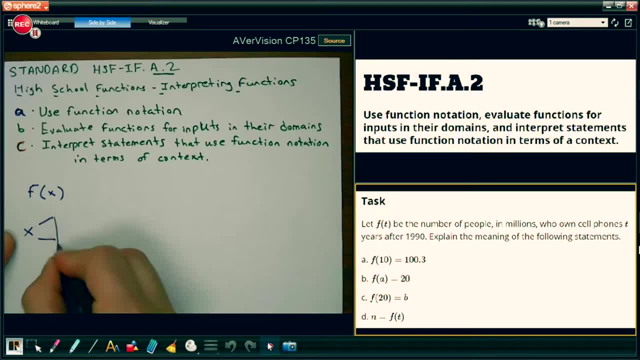 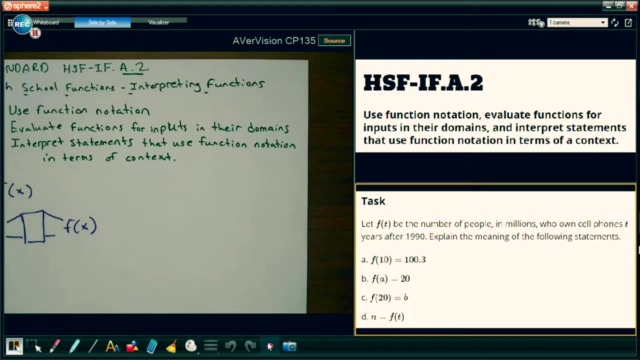 and if we put our input into our function machine, the output is going to be some f of x. Now we have to evaluate functions for inputs in their domain. So we said: and for these, If we have a function like f of x equals 2x to evaluate. we would create a table, put our inputs on the left and our output after the evaluation can come out on the right. 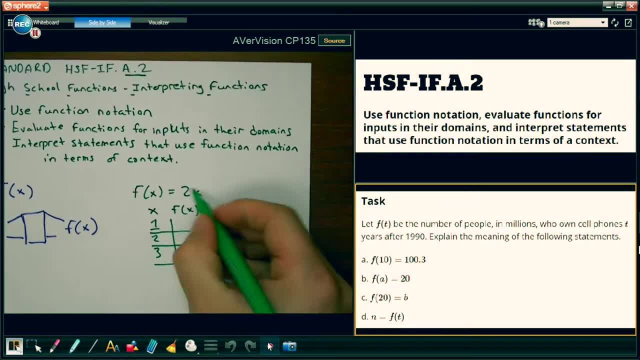 So I put 1 into 2x as my input and I get 2.. If I put 2 into f of x as 2x, that would be my table. That's a simple evaluation of functions as inputs in the domain which is x. 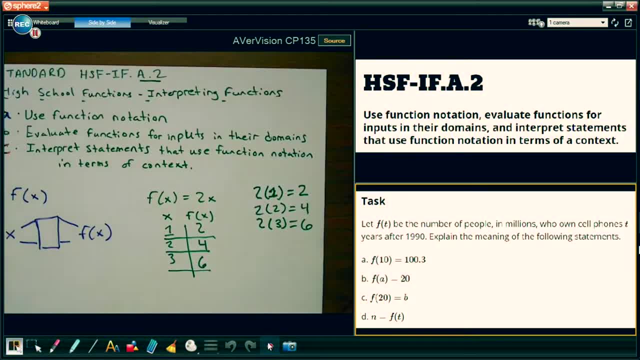 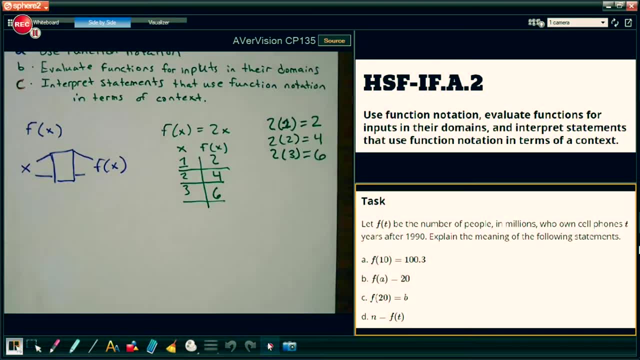 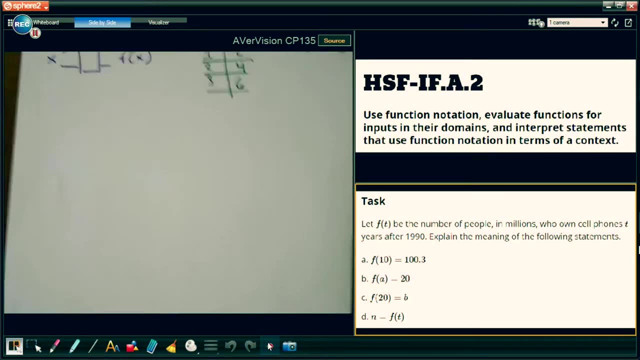 Now C. the third part is a little bit trickier, Interpreting statements that use function notation in terms of context. So I've set up a problem on the right under task. It says: let f of t be the number of people in millions who own cell phones a few years after 1990.. 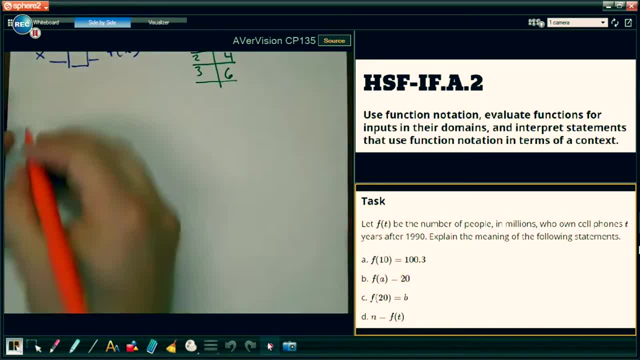 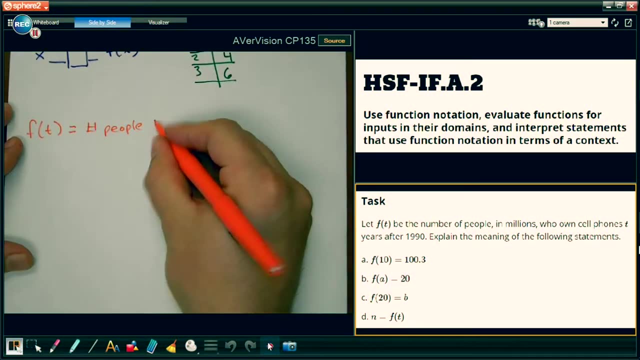 Explain the meaning of the following statements. So f of t Is the number of people who have cell phones a few years after 1990.. So I look at this statement and t years is the t that we'll take as the number of people who own cell phones a few years after 1990.. 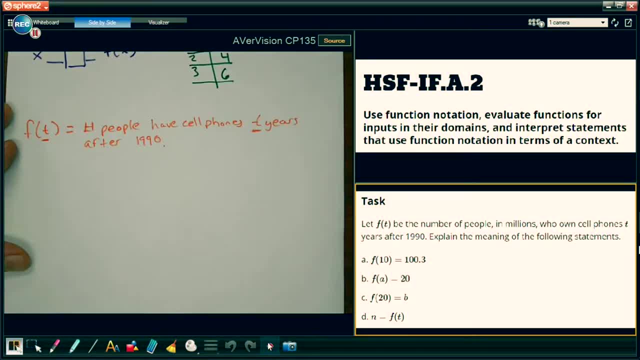 As an input as part of the domain of my function. So the first problem is: f of 10 equals 100.3.. I have to evaluate and interpret this statement using function notation, in terms of the context. So the context is that the domain inside of the parenthesis of the function is equivalent to t, which is the number of years after 1990..